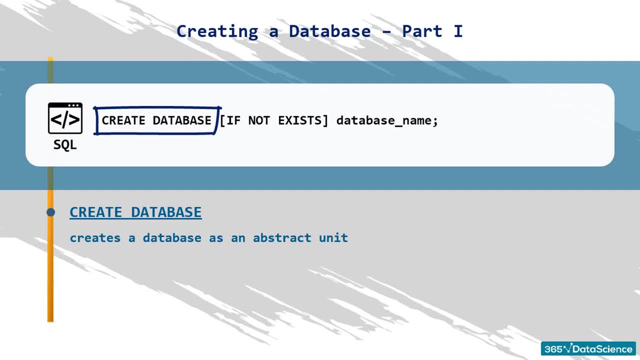 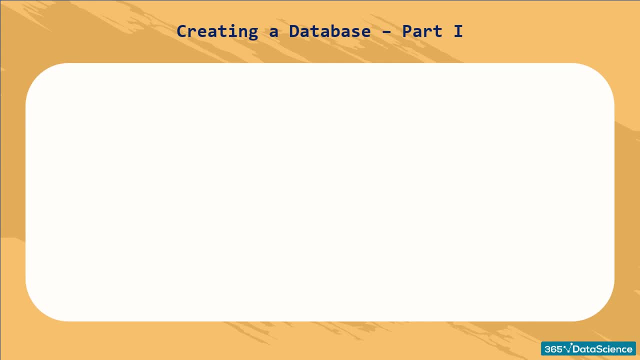 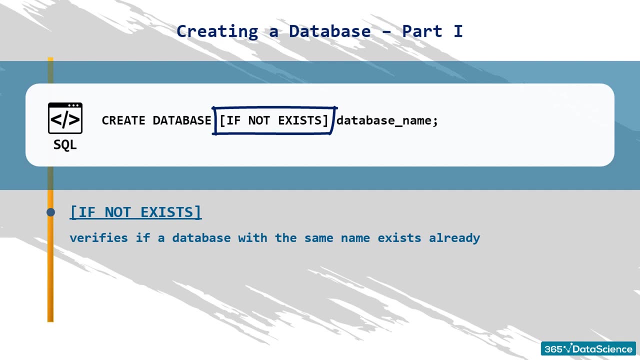 represent an object ready to be filled with information. Think of it as creating a canvas on which you would be able to draw your relational schemas later. IF NOT EXISTS, will verify if a database with the same name exists already. If it does, this will impede us from creating a database with the same name. 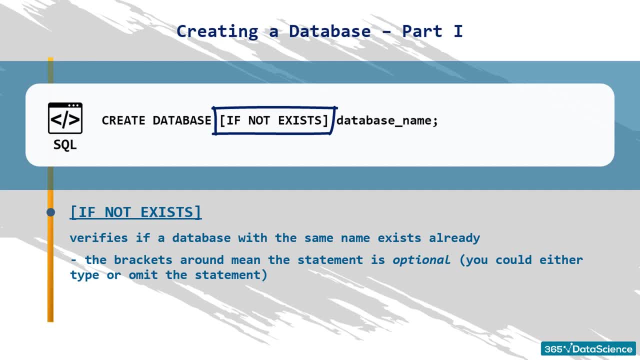 The brackets around indicate that the statement between them is optional. in the syntax, Optional means you could either type or omit the statement. This is the situation with: if not exists. Even if you don't include it, the code will run anyway. Nevertheless, we advise you to always use it, because it allows you to avoid potential 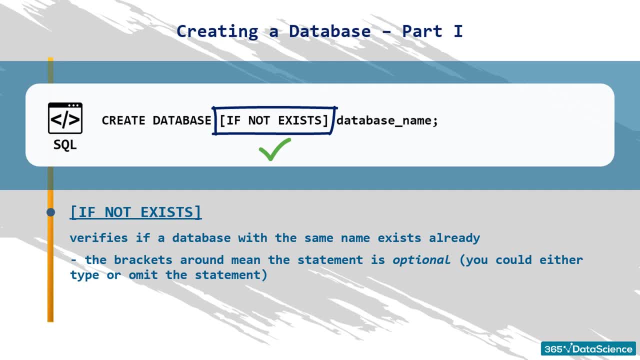 errors. when working with large amounts of data, It is good to build the habit of attaching this phrase straight after the CREATE statement. Next, we will have to specify the name of the new database. We strongly suggest you give a name that is short but at the same time as related to 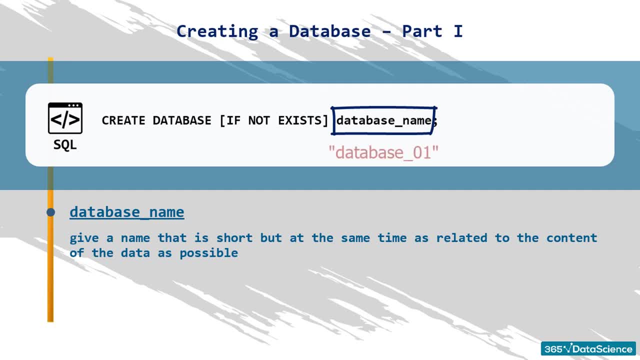 the content of the data as possible. Try to avoid assigning names like database underscore zero one or database underscore about, underscore sales, underscore in, underscore new, underscore york. In our case, the data we will work with is about the customer sales registered in a company. 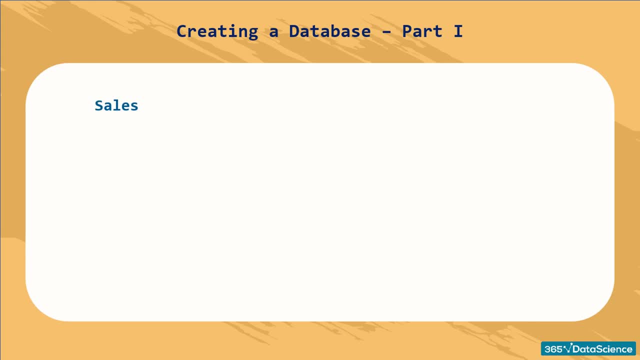 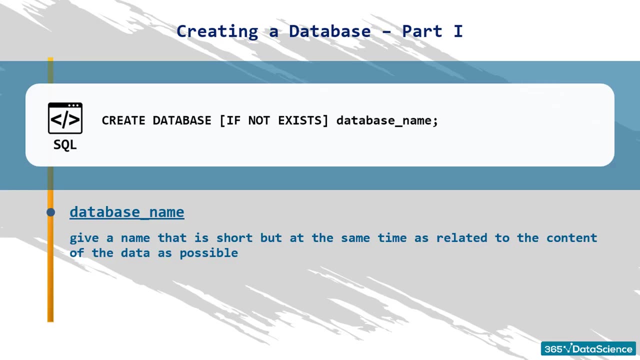 For this reason, we will call the database Sales. Whether you use uppercase or lowercase letters only, or both, it's the same for SQL. The SQL code is not case-sensitive, Neither when assigning names of objects nor when writing queries. Otherwise, in this element, the quotes are optional. 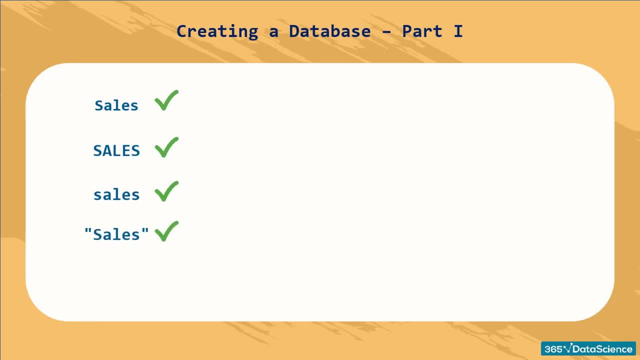 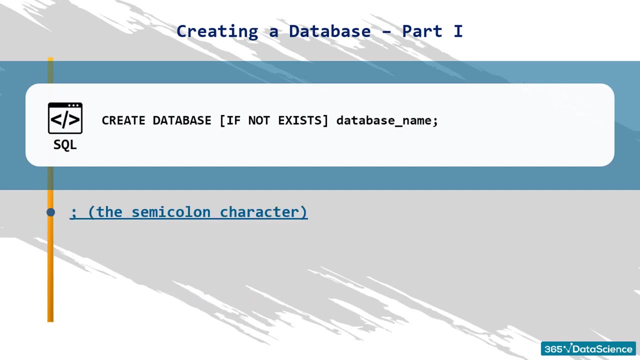 You could either say Sales within quotes or without using any quotes. It makes no difference. Finally, you should always end your statements with a semicolon character. It functions as a statement terminator. Yes, it is often true that your queries will run properly without it. 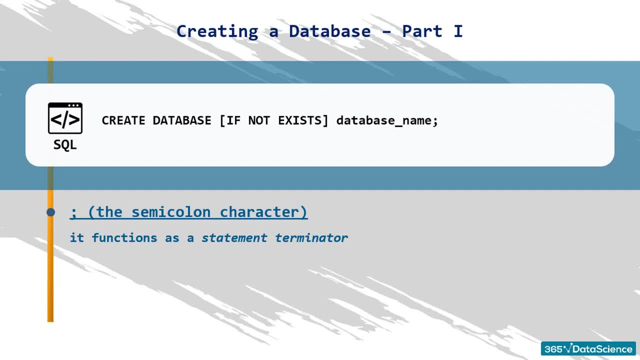 But this is not the point. In longer scripts, when your code contains more than a single statement, the semicolon is indispensable. So please try to end your statements with this character. This will not only help you avoid errors sometimes, but will also improve the readability of your 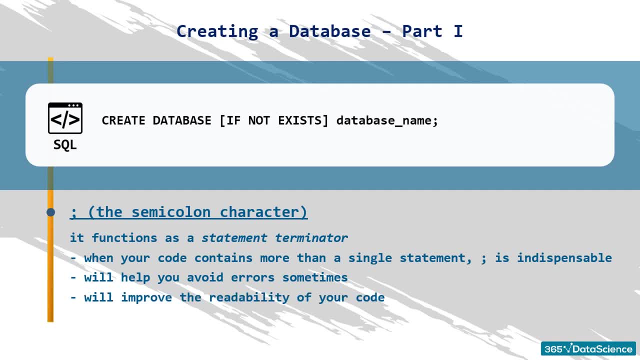 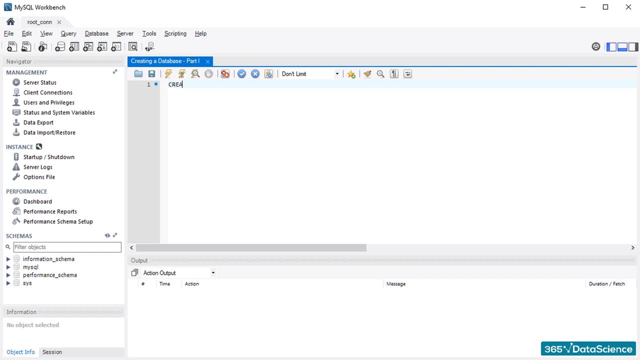 code. Ok, so I guess we are ready to type down our first query and run it, aren't we? Let's type: create database if not exists without brackets: Sales, keeping in mind that we are allowed to omit the quotes without any problem. and 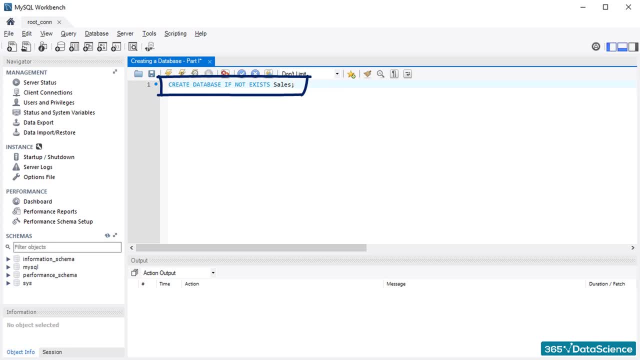 similarly the quotes. So let's start with the first query. This is the first query. Let's see if we can get it right. Let's type in a semicolon Now. it is important to note that this entire line is nothing but a piece of text until 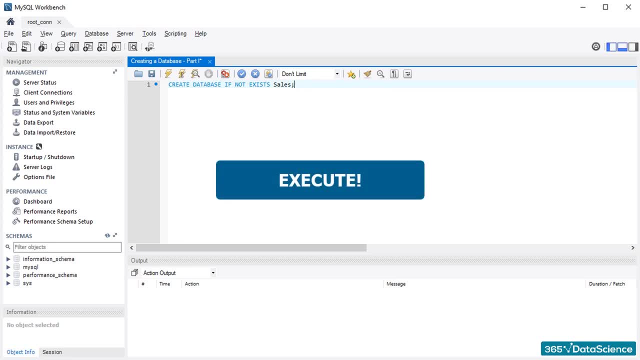 you execute it. To execute or run a query, you must press this lightning symbol. The alternative is to implement the shortcut combination Control-Shift-Enter. So what are we waiting for? Let's press this button and see the output of our work. 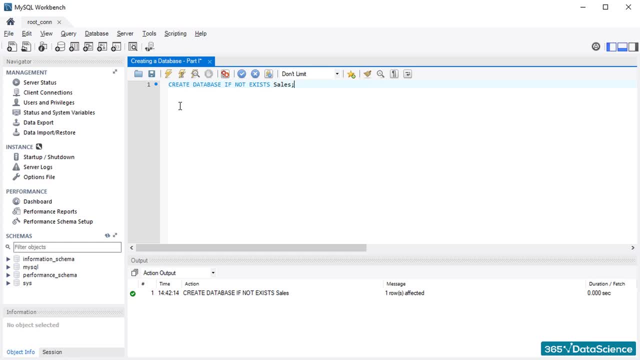 At first sight, it seems nothing happened. This is not the case. This is not true, though. When new databases, schemas or tables are created, we always need to refresh the content in the Schema section at the bottom left part of the screen. 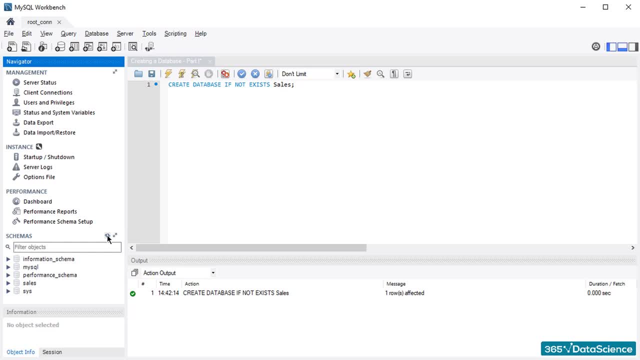 By pressing this little button here, Ha, The Sales database is ready for use. Great, Please remember that you could have achieved the same output if you had used Create Schema instead of Create Database. Considering that database and schema are practically synonyms, this seems like a logical alternative. 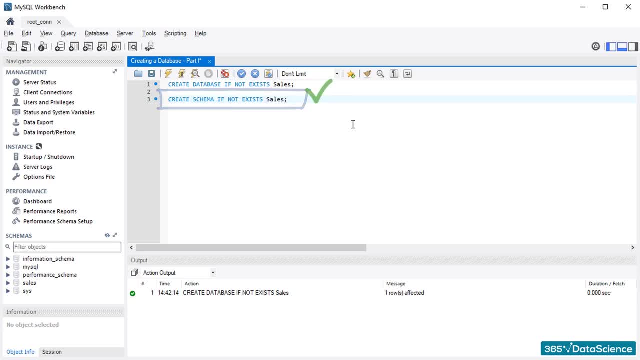 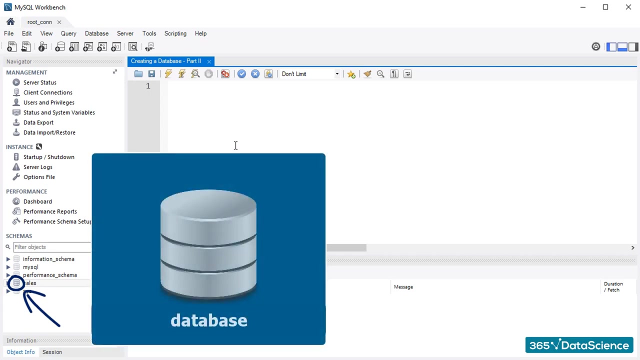 Right. Well, we just completed our first task: creating a database. Congratulations. In this video, we will look at the MySQL Workbench interface in more detail, as it can help us manage our database better. The symbol located before the name- Sales- indicates us that the object in question is a database. 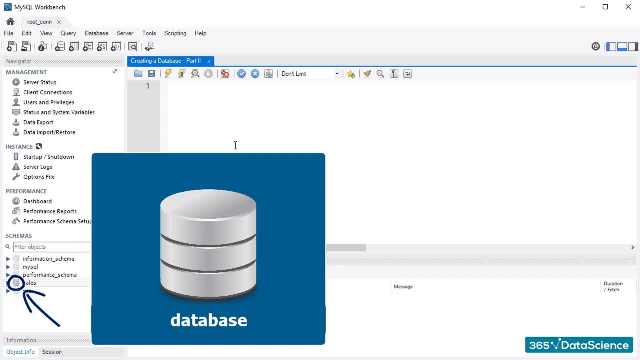 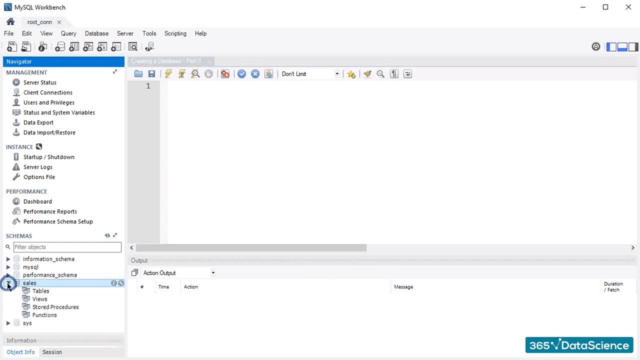 You've seen it before, haven't you? It stands for a database. Moreover, by pressing this miniature triangle, we see how this database can be broken down into four components – tables, views, stored procedures and functions. Since we have not created any of these for the moment, nothing will happen if you click. 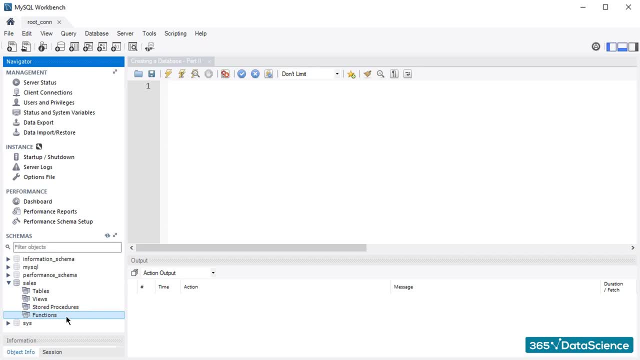 any of the respective names. It is important to be familiar with this little symbol that appears when you hover above the name of the database. It is a feature of the MySQL Workbench you will love when you fill in your database with data. Once you press it, a new tab containing information about the database will open in the right part. 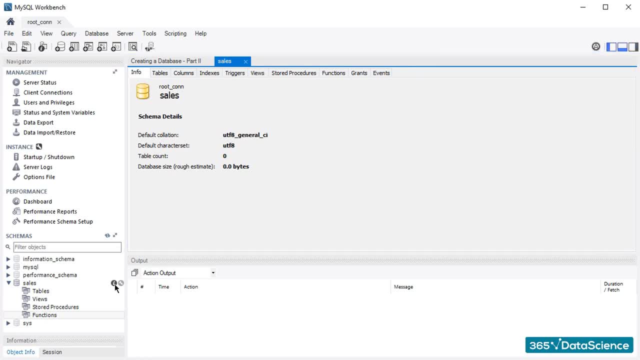 of the screen, Although all these fields are currently empty. when we fill our database with information, we will be able to inspect its tables, columns, indexes, triggers, views, stored procedures, functions and grants in a great level of detail.